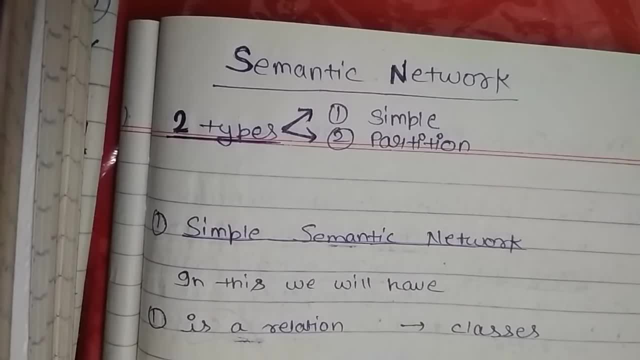 Semantic network is of two types And in exams they will ask you to construct a semantic network. Okay, so it is of two types. First type is simple semantic network and second type is partition semantic network. And now in this video I will explain you how to solve simple semantic network questions, but how you can create it. But firstly I will tell you some basic things to solve this question. Okay, simple semantic. 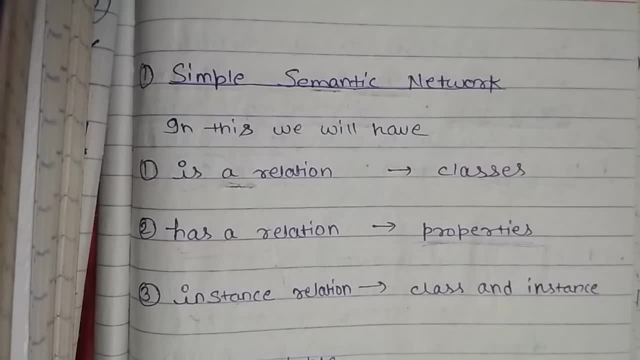 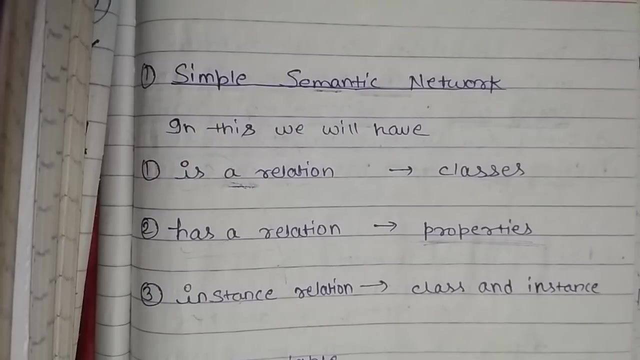 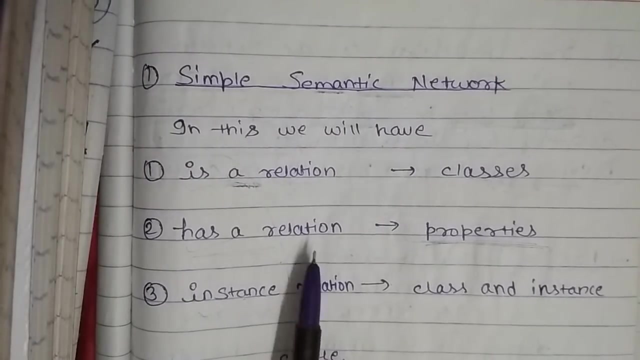 network is kind of easy as compared to partition. In partition semantic network you have to consider some things, But here you can make your own story. See, in this we will have is a relation, Is a relation exists between classes, Okay, between two classes. we have is a relationship, And we have has a relationship in here, and which is used to represent properties of classes, Okay, properties of 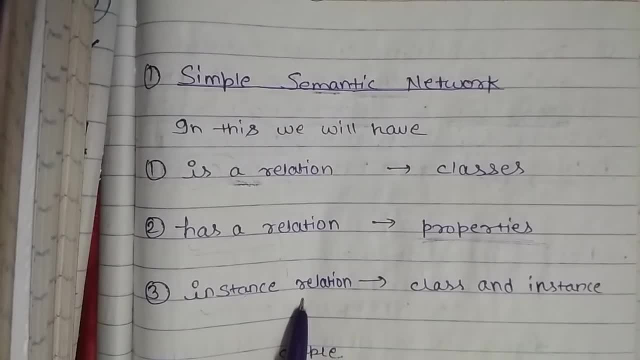 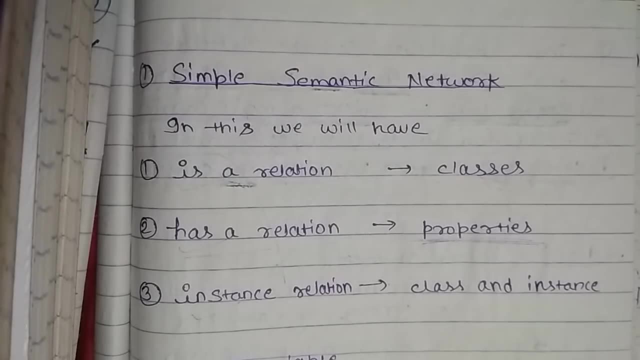 a class. Okay, and we have instance relation. Instance relation is used to represent class and instance. Suppose we have a class and we are giving instance of that class, So this relation will become as instance relation. And if in exam they have told you to construct simple semantic network, then you must have to include all of these three relations to solve that question. Okay, you must have to include. 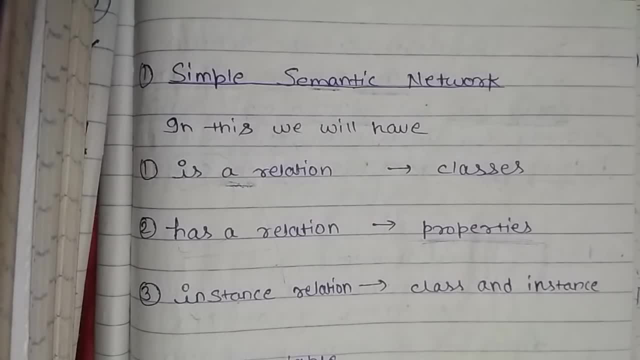 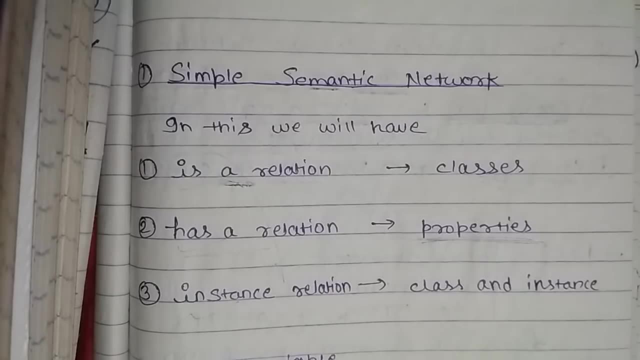 Okay, so If you will not include, then they will cut your marks. So these three relation must have to be there in your solution: Is a relation, has a relation, instance relation. And now to make it more clear to you about: is a relation, has a relation, instance relation. 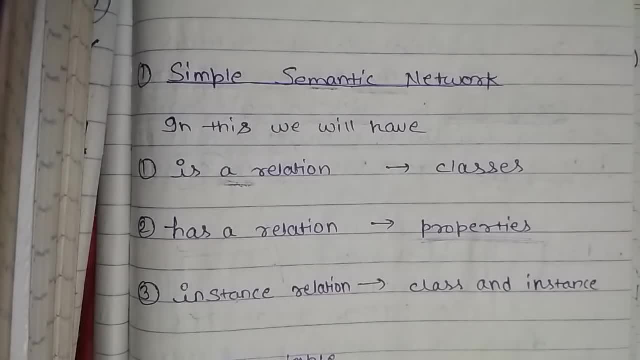 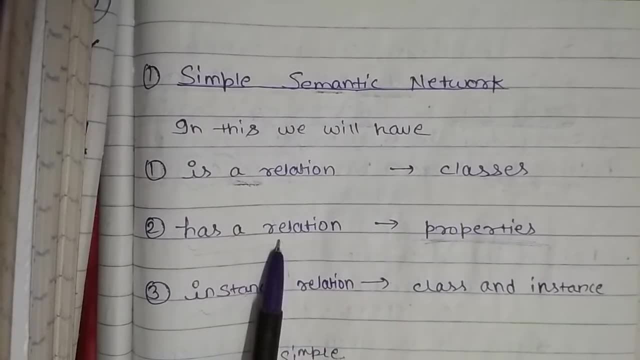 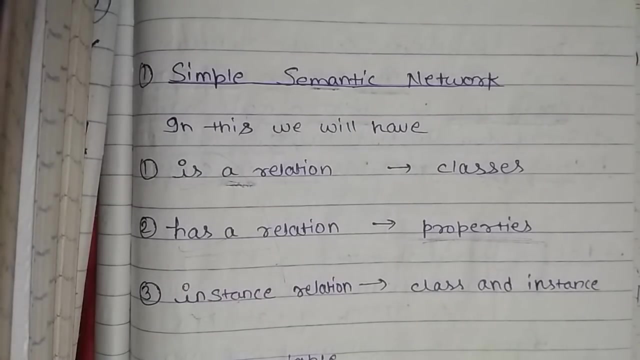 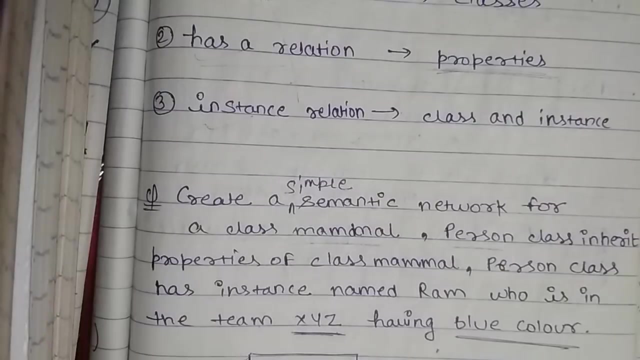 I will give you a simple example. okay, to solve simple semantic network. So is: a relation exists between classes, has a relation exists between properties, properties of those classes, instance, relation exists between a class and an instance. So now I will tell you an example. 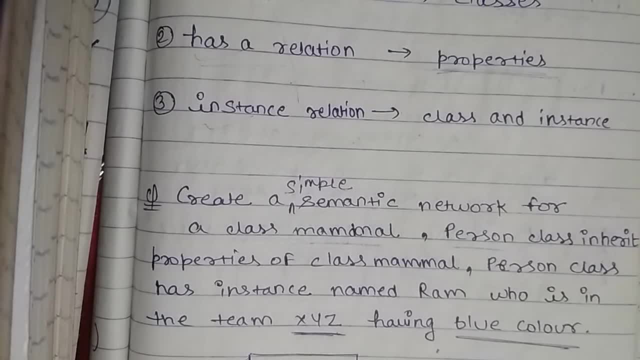 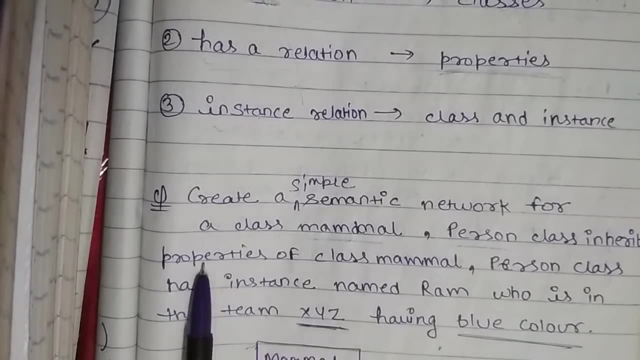 Suppose this is a question in which they are asking you to create a simple semantic network. Create a simple semantic network for a class mammal. Person class inherits Property of class mammal, So this class is inheriting property of class mammal. 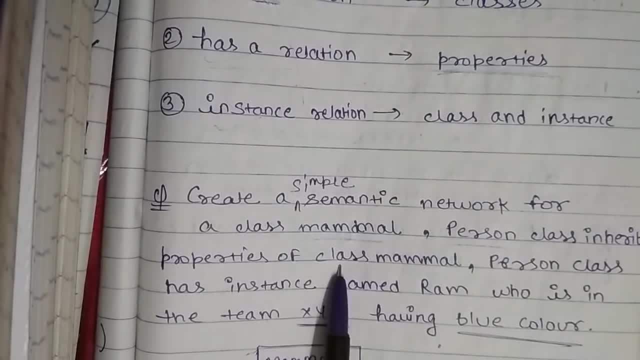 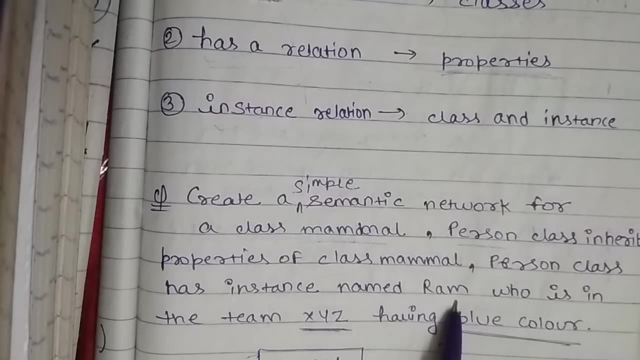 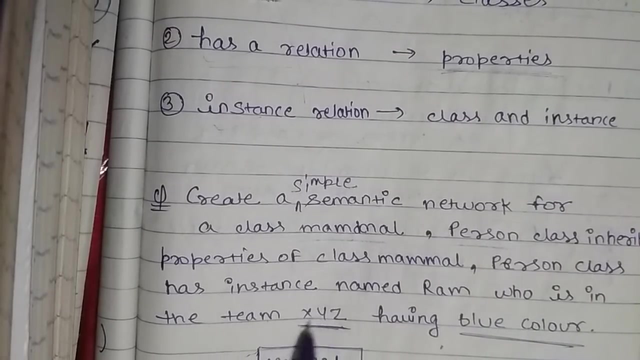 So this is child class, this is its super class or parent class? Person class has instance named Ram. okay, Instance of person class is named as Ram, who is in the team XYZ. Suppose the team name is XYZ and Ram is in that team. 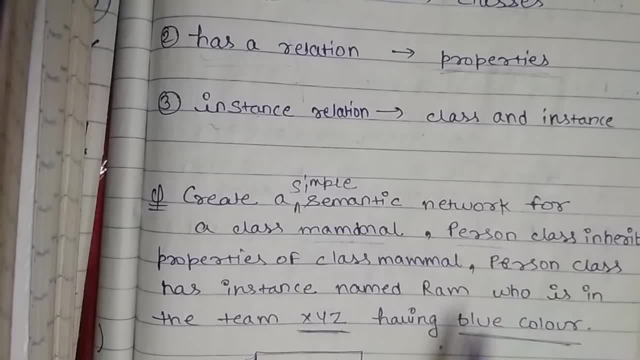 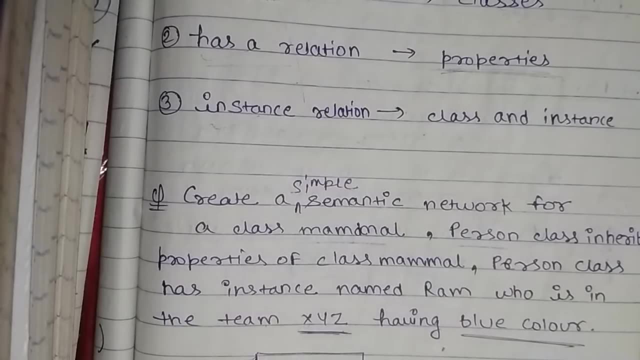 Ram? what is Ram? Ram is an instance. Ram is an instance of person class and the team is having color as blue. So this is a property. So everything is mentioned in the question and if you are not getting the properties, relations and is a relation, has a relation, instance relation. I will explain you it now. 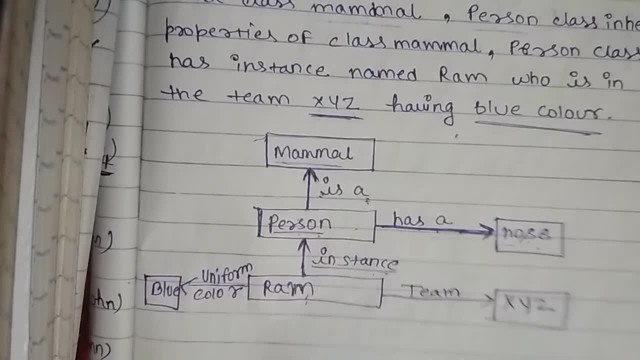 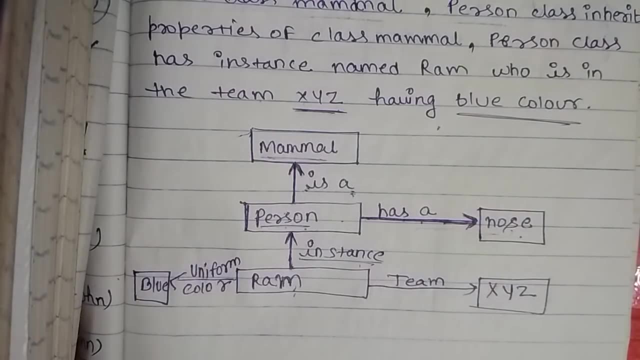 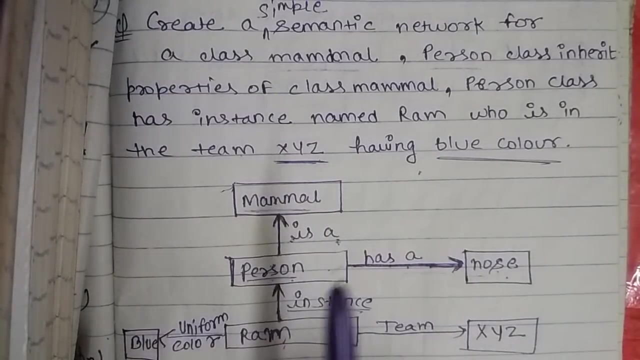 So the solution for this question will look like this: okay, see, but just see the solution first. I hope you will get the solution, but I will explain it to you now. See this thing: person class is inheriting properties from mammal class. 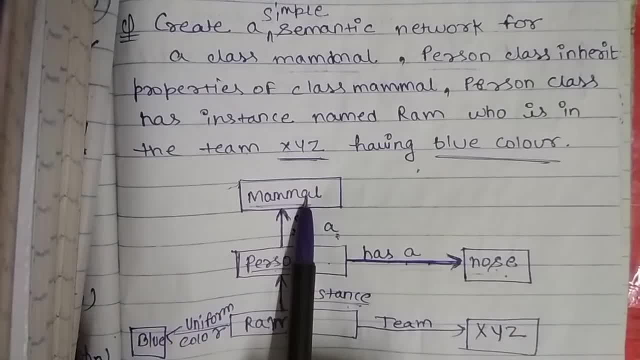 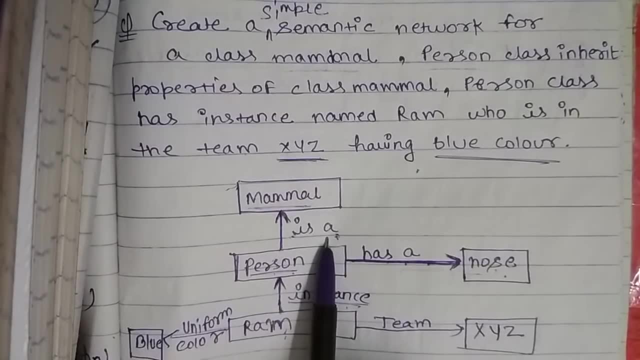 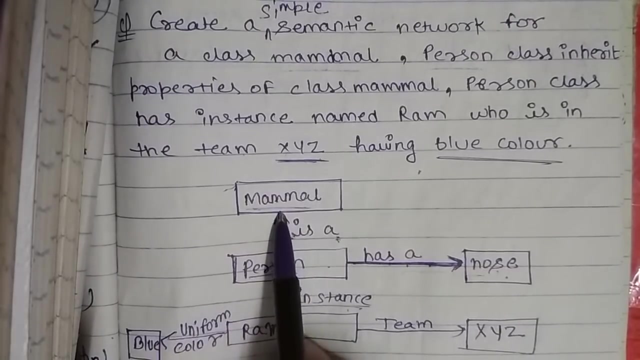 Person class will become child class, mammal class will become parent class and the relationship between two classes is is a relation. is a relation is used to represent relationship between two classes and the. you have to use arrow like this: The. this arrow will represent the relationship between two classes. 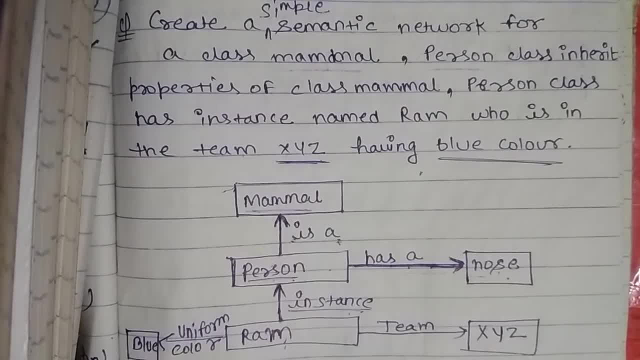 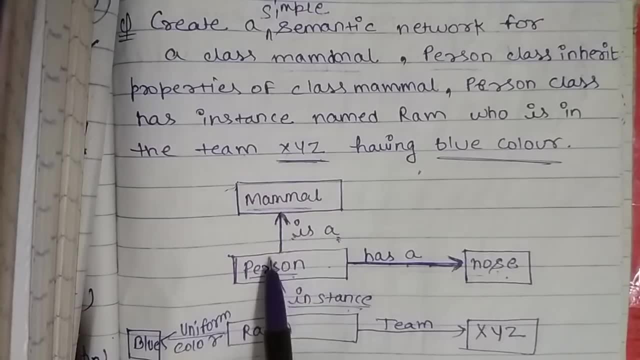 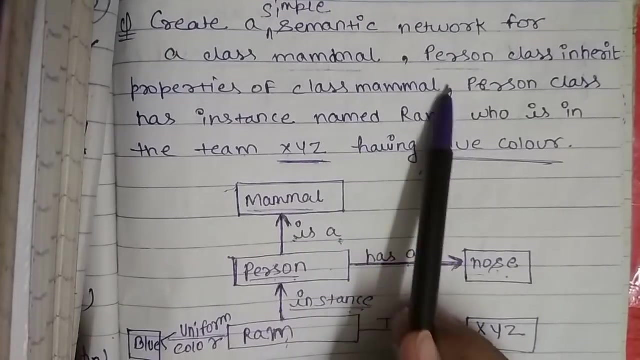 So arrow will go from this here to here, because it is a, is a relation and it is a child class. So to represent child class you have to use arrow like this. Arrow will go from child class to parent class. okay, So person class is inheriting. person class inherits property from class mammal. 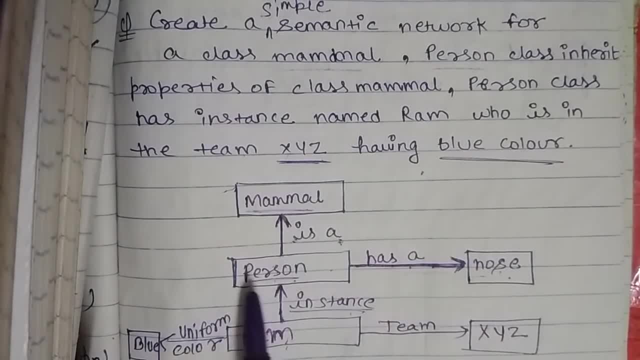 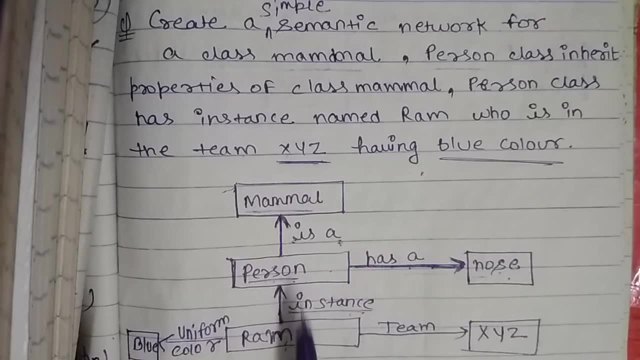 Person class has instance named Ram. You can give arrow here or here. I am giving arrow, as here, Here, Here, Here, Anywhere you can give arrow. I am writing here arrow, as like this: Person class has instance named Ram. 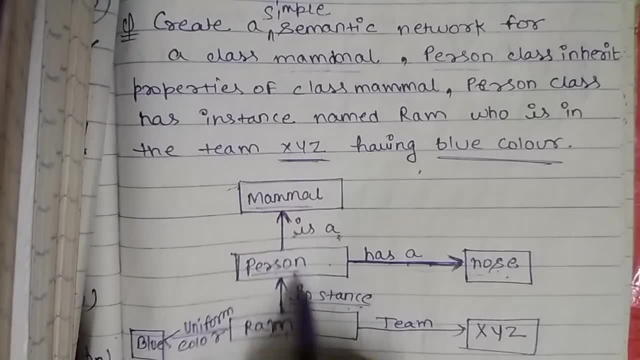 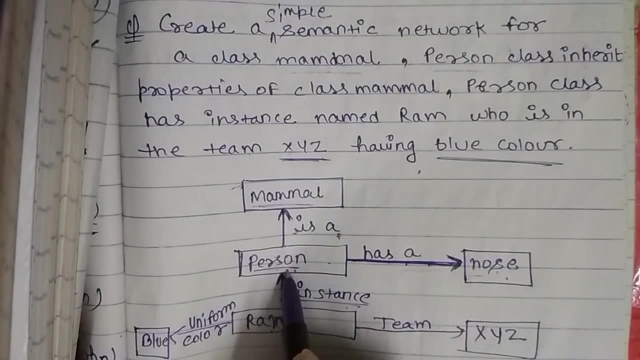 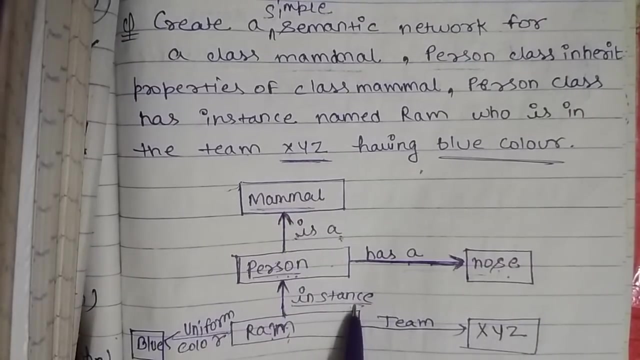 So Ram will become instance of person class and this is a instance relation. So write here instance and give arrow from instance to the class where it is inheriting property. So here you have to write: is a relation, here you have to write instance relation, because 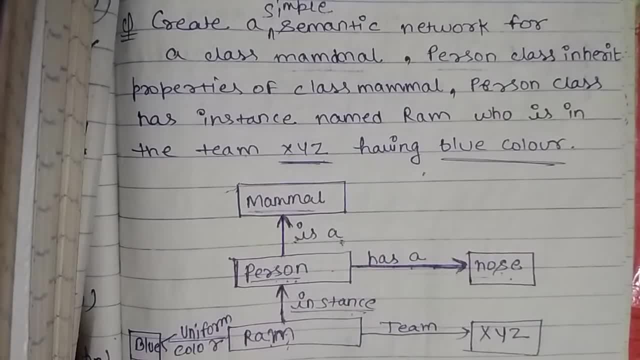 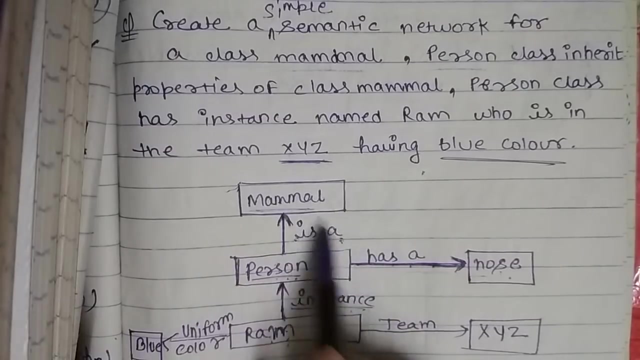 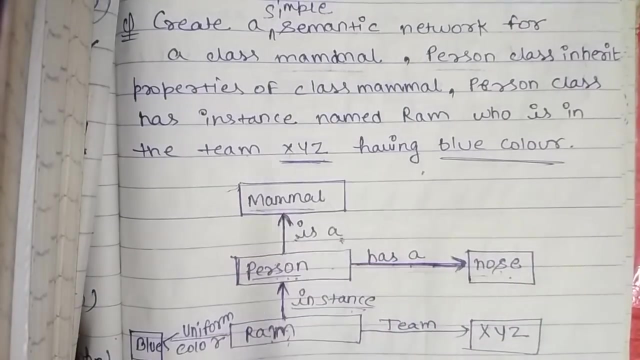 Ram is instance of instance of parent class. Now, just ignore this for some time. Just, I have written it for some more new points, but just ignore it. okay, Just see these three things first. After that they are saying: that instance named Ram, who is in the team XYZ. 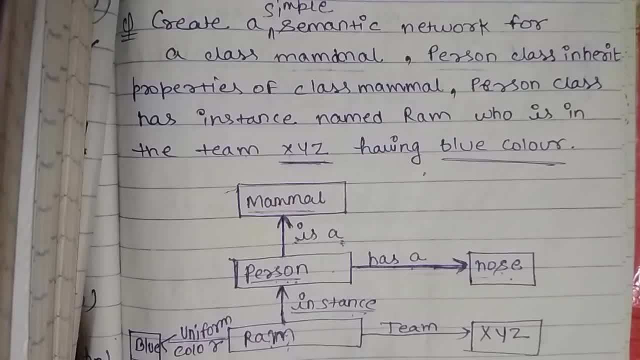 So Ram is in the team XYZ, So it is not any relationship. It is not any relationship. It is not, is a relation, has a relation or instance relation. So just symbolize it in a shorter way. So write here: team XYZ. 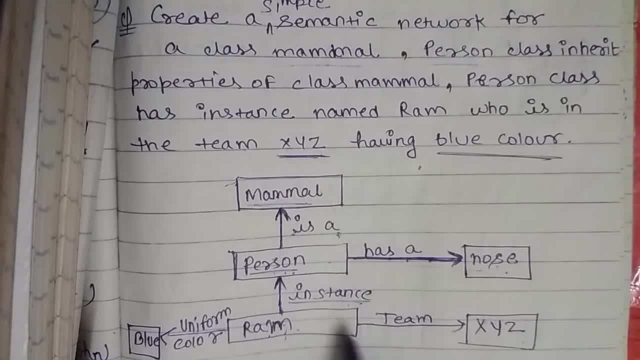 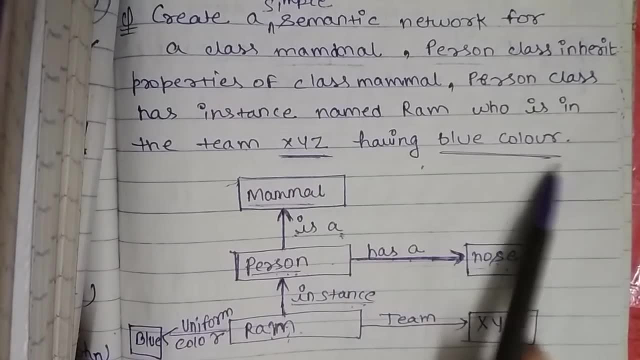 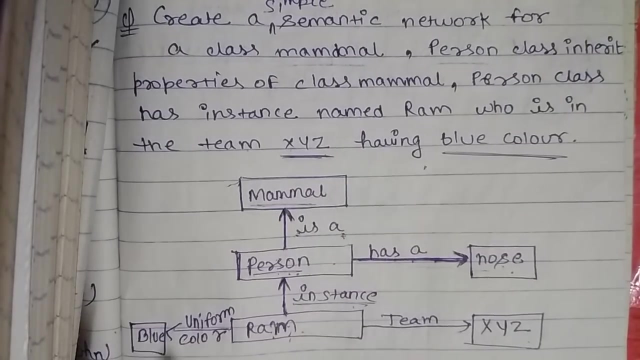 It will represent that Ram is an instance of person class and it is in the team XYZ And they are talking about color of team XYZ, which is blue color. So this team is having a uniform color, which is blue. So just write here blue and represent it like this. 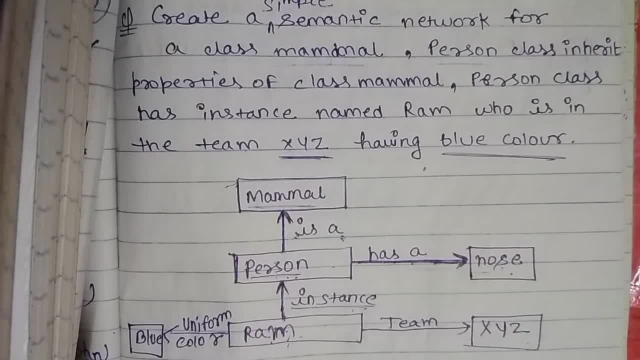 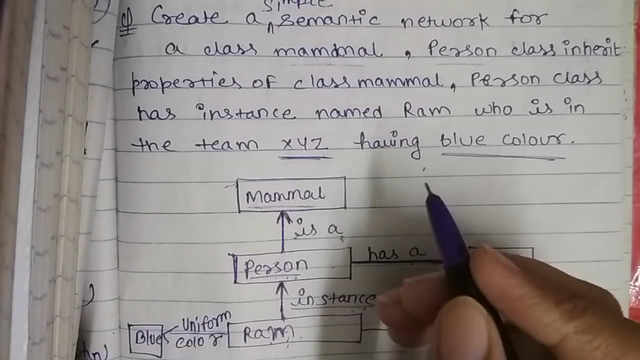 Okay, So I hope you got this. Now in this question they have not told you to draw has a relation. They can do that, but you have to. you should represent it also. So to represent this: suppose they have told you that who is having blue color and person. 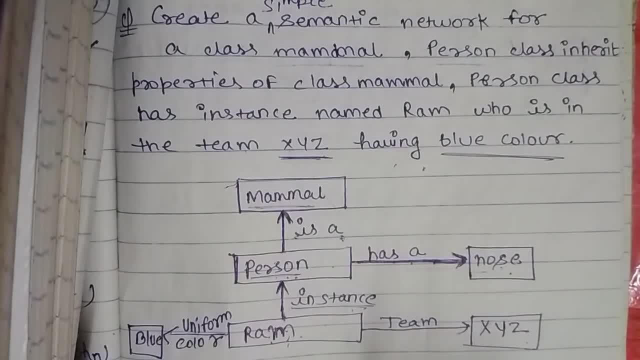 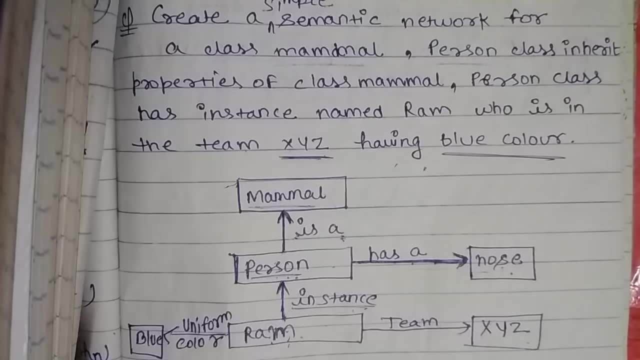 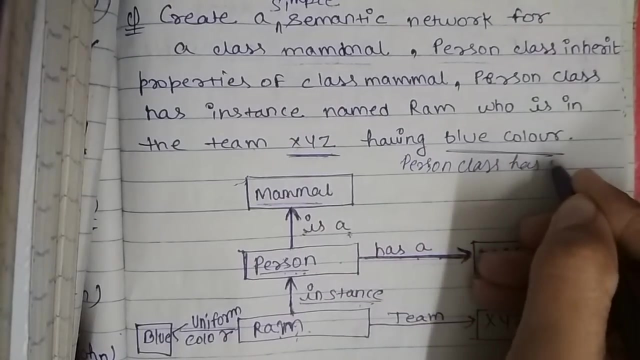 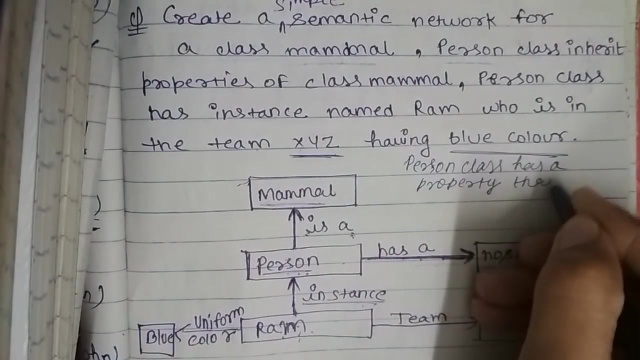 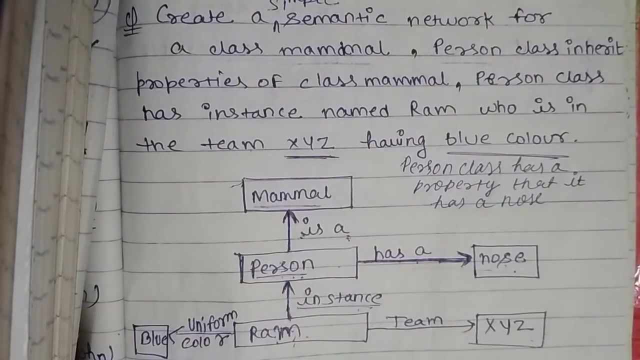 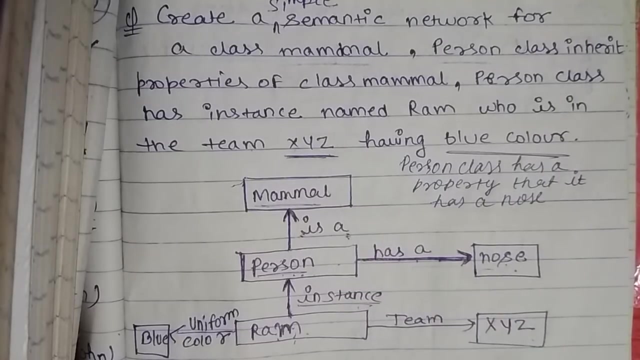 person class has characteristics as a person- Okay, nose. so this is a. has a relationship. they will ask you in question, that person class has a property, that it has a nose, it is having nose or it contain nose. they will say you, so you have to write it as person has a nose, okay, so it is a has a relation which is used. 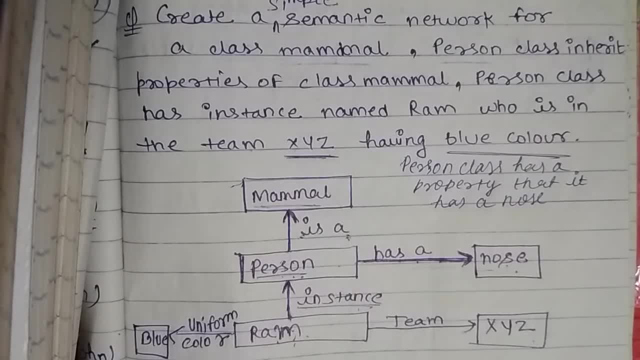 to represent properties of a particular class. here the particular class is person class. okay, so they just forgot to mention this thing, but i have included it also. so this is the simple semantic network example and in exam they will ask you any question. and just remember that you have to write it as person has a nose. so you have to write it as person has a nose. 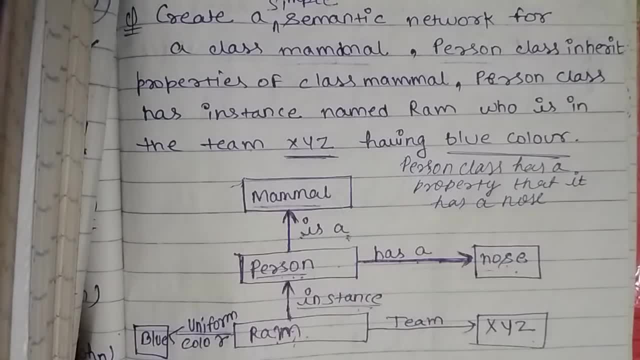 and just remember that you have to include all three: relation is a relation, has a relation, instance relation- in this way only.